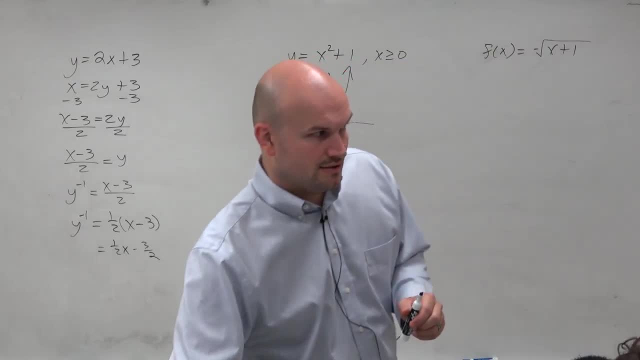 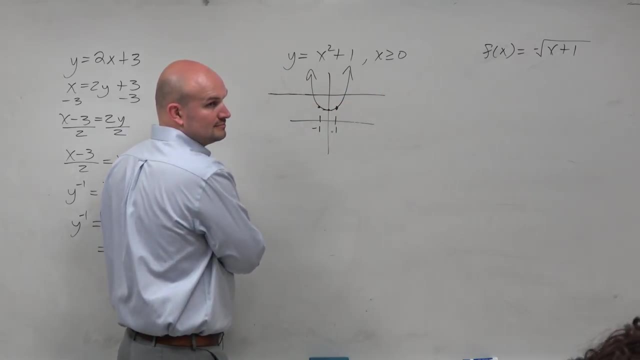 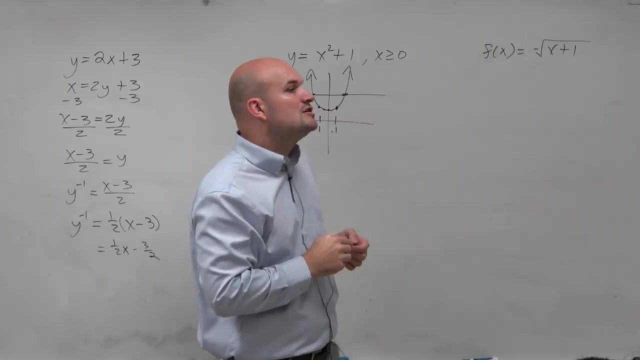 but it's not one to one. Another way to look at that, another way to determine if something is one to one, is to use the horizontal line test. So something is one to one if it passes the horizontal line test. This does not pass the horizontal line test. So therefore the 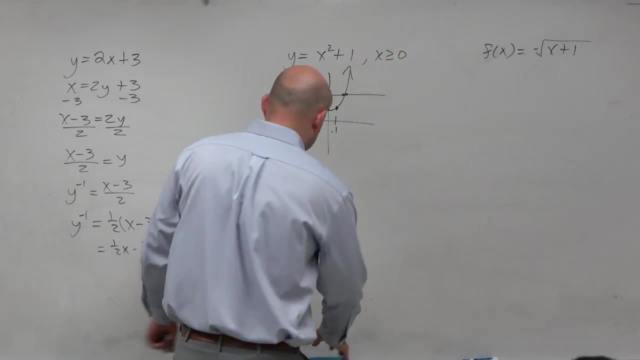 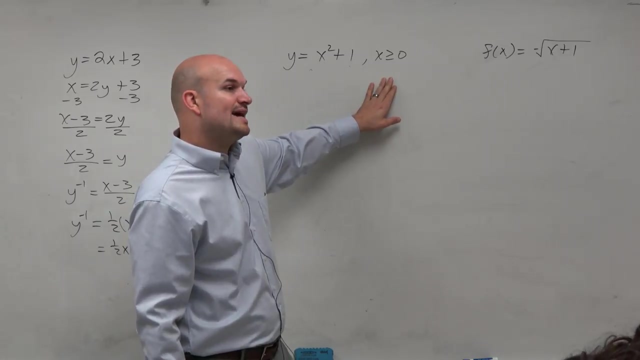 inverse is not a function. However, In the example that I showed you earlier, the inverse was not a function. However, that we are doing, there's been a restriction placed on this for only x values greater than 0. And, oh, we've been practicing restrictions, right? So let's go ahead and do that again. 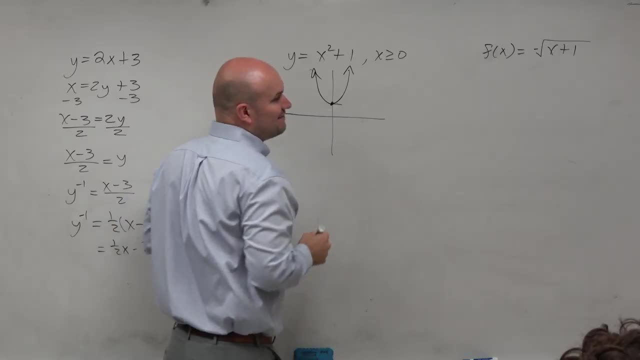 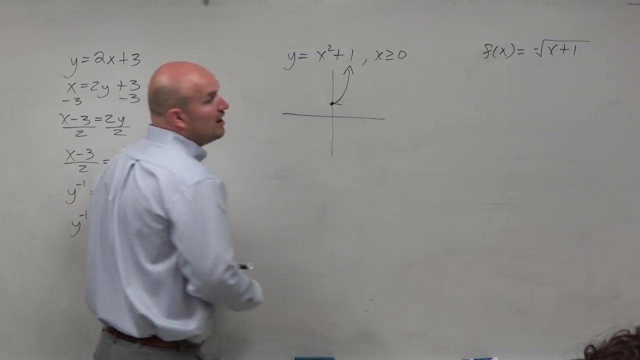 So I have x squared plus 1, but I only want to graph this for x values that are now greater than or equal to 0.. So this graph really just looks like this: Is this now 1 to 1?? Is it now past the horizontal line test? Yes, So now I can find the inverse. So now I can find. 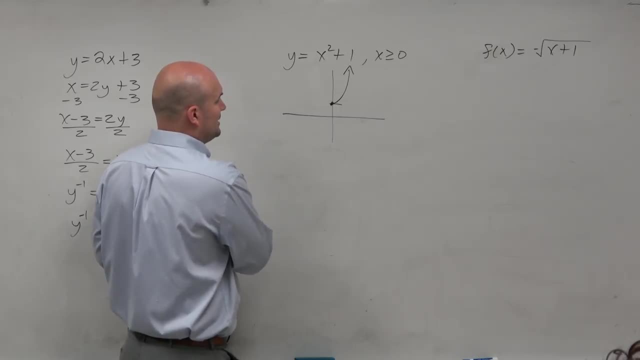 the inverse of this And I'll show you what I mean. So again, kind of steps we have. This is y equals. So we're just going to set x is equal to y squared plus 1.. Swap the variables. Now we've got to solve for y Subtract 1, subtract 1.. x minus 1 equals y squared Undo. 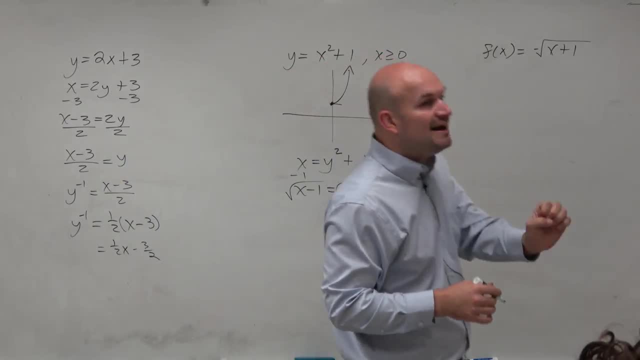 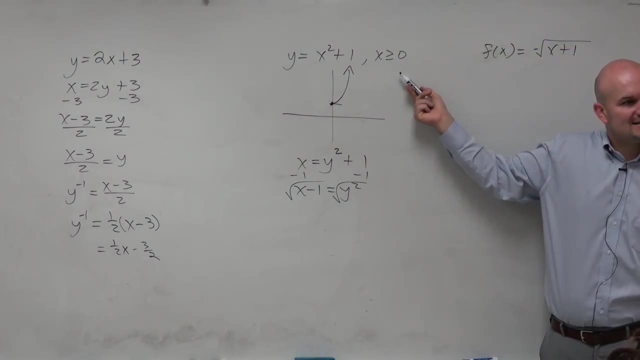 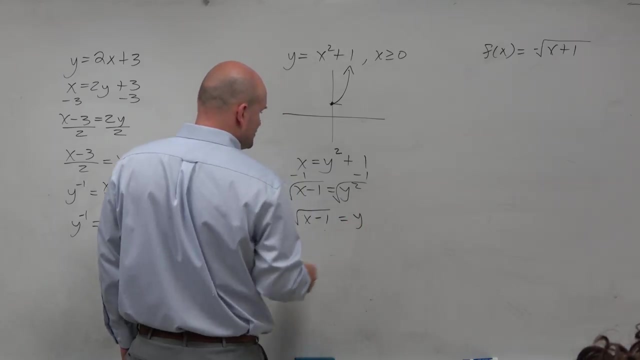 squaring by taking the square root. Whenever you introduce the square root, you have to include plus or minus. But in this case do we have to include minus? No, because we only want the positive version. So therefore we have positive x minus 1 is equal to y Or y inverse is equal to the. 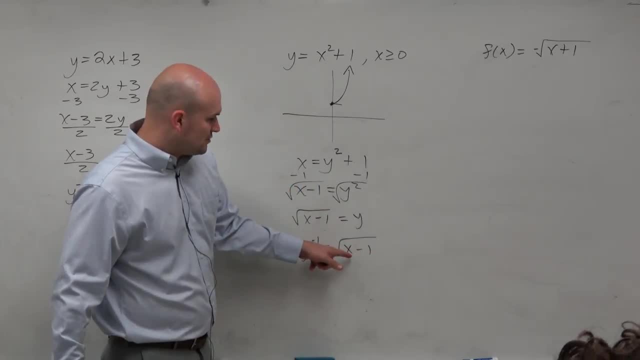 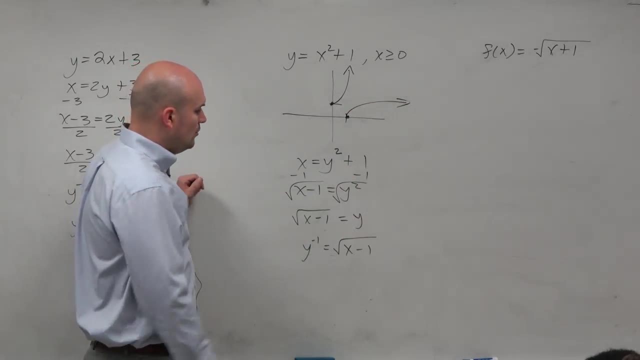 square root of x minus 1.. And let's just go and graph that. If I was going to graph the square root of x minus 1, it would look like that, right, What if it was plus or minus? What would the minus of that look like? That would be a reflection about the y-axis. Do 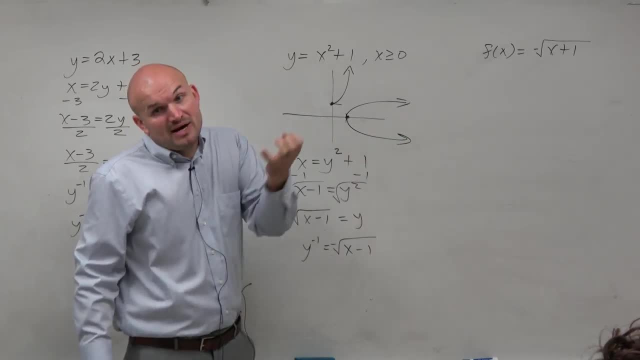 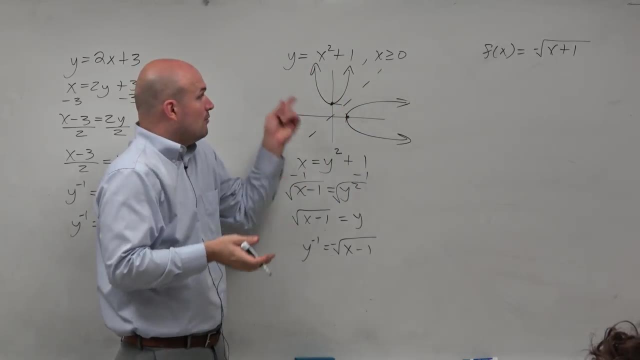 you guys see how the plus or minus makes that not a function, Right? That's why it's important, important to have something one-to-one, Because look you guys, that works. The problem with it if it's not one-to-one, the inverse is. 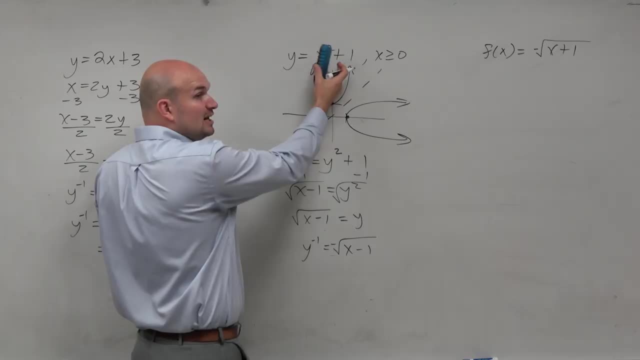 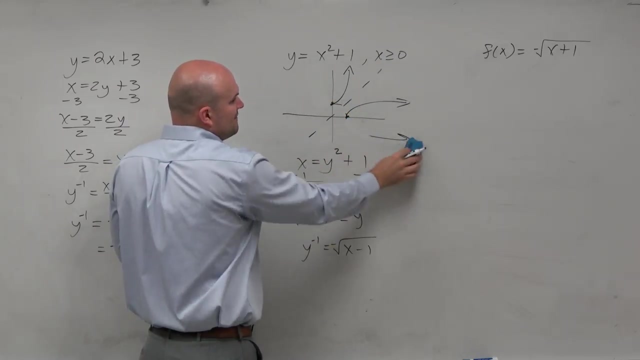 not a function. So that's why it's: either you're going to get a problem like this and say, hey, does it have an inverse? And you say, no, it's not one-to-one, Or it will be restricted and it'll say: find the inverse.